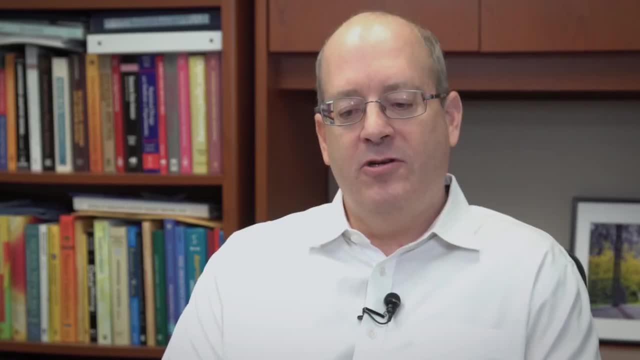 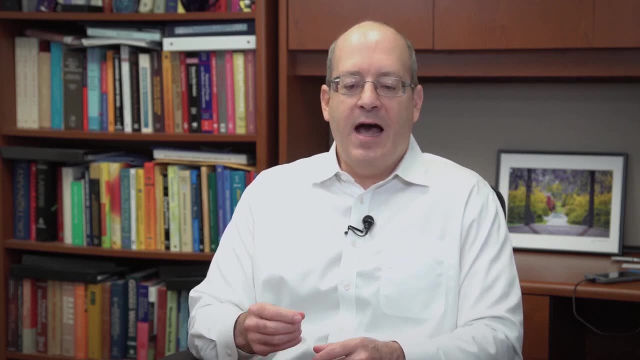 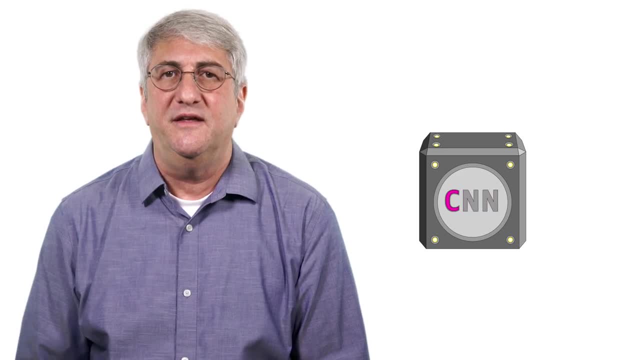 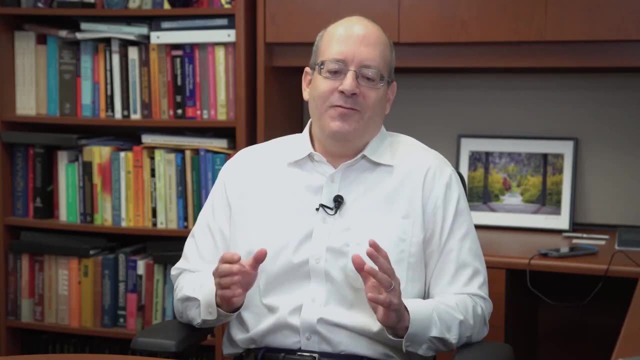 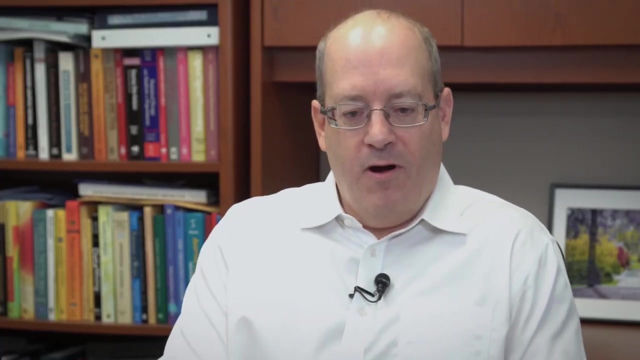 Let's say we have a building block A, B, C and D. That's where things get difficult. Let's say we have a weird anything-or-not All county's building blocks. you just S over both places and you have to Think of it like this. 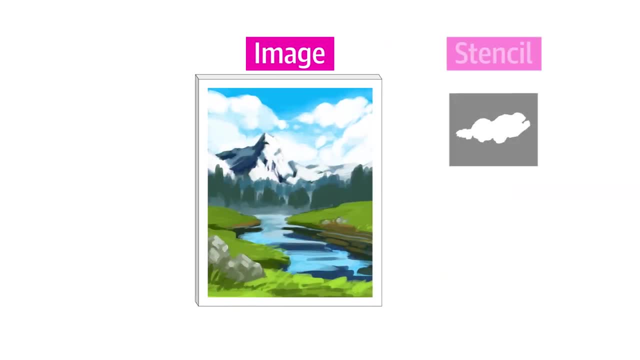 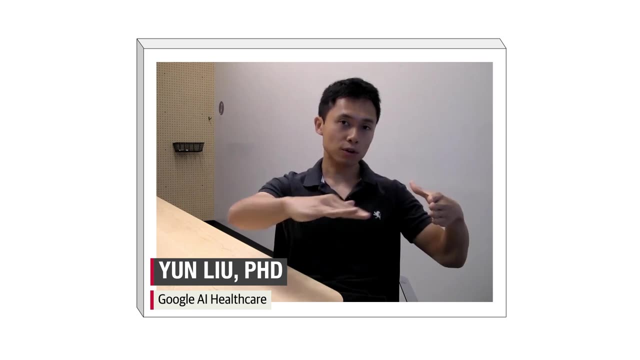 You have a drawing, That's the image, And you have a dois stencil- That's the filter. You take that stencil and pass that stencil over that, that drawing that you have, and as you do that, you'll see that some parts of the 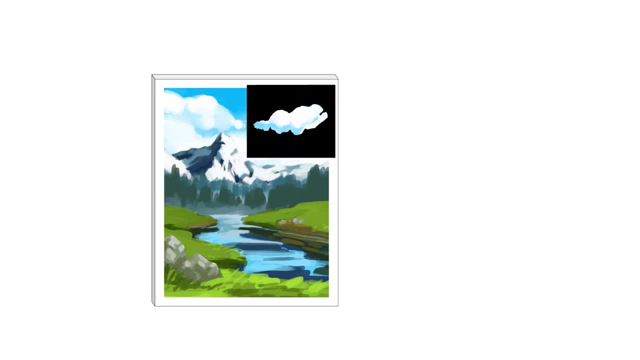 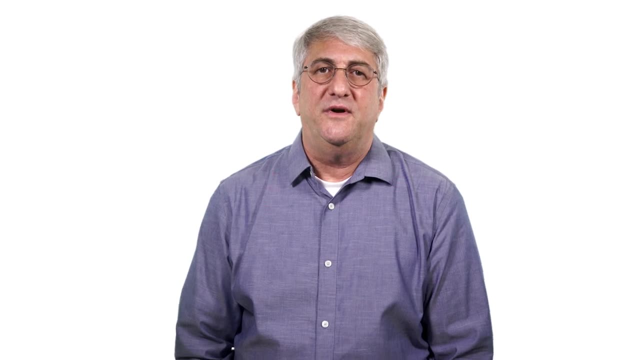 drawing become more visible than others as you do that right, And that process of sort of sliding that stencil across this drawing is essentially the process of convolution. Now that we've explained what a filter is and introduced the concept of convolution, let's use an analogy of written language to 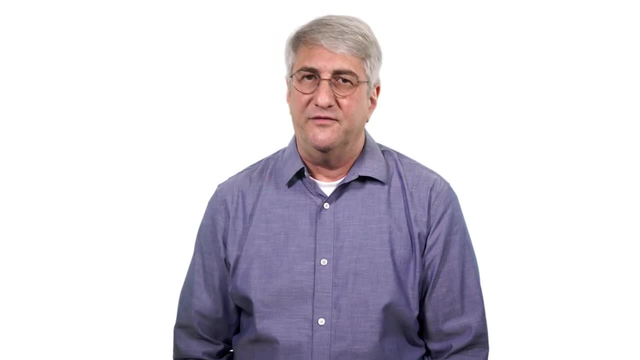 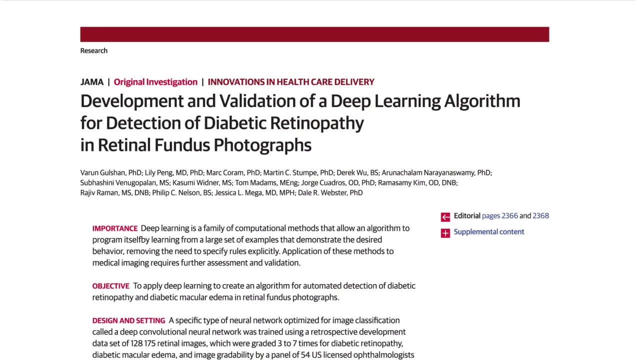 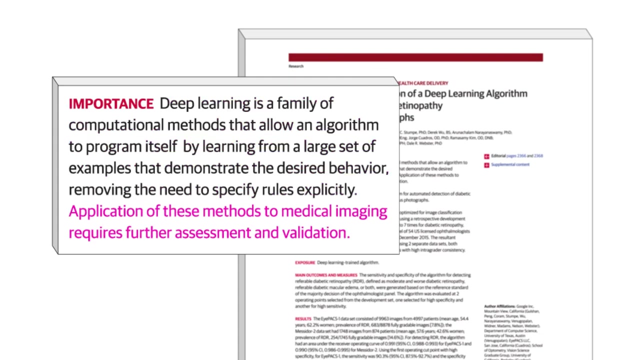 understand the relationship between the filters and the hierarchical structure of the layers in a CNN. We will simplify the explanation by using an analogy. The analogy is a written document. In order to communicate through writing, we organize it as a series of paragraphs which are composed of sentences, Those 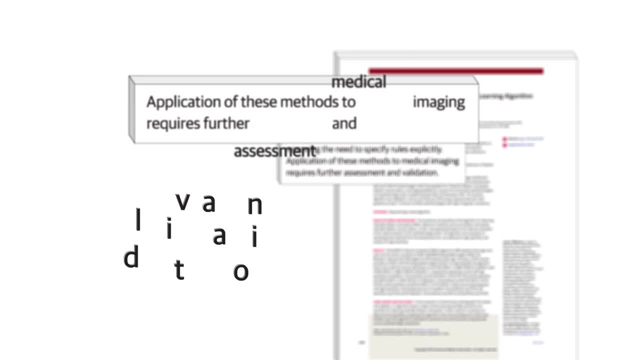 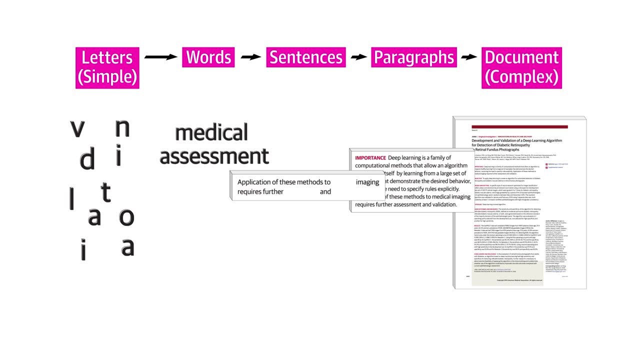 sentences are composed of words and the words of letters, So reading a document requires assessing the relationship of letters to one another in increasing layers of complexity, which is a kind of deep hierarchy, like the hierarchy of conseguir orden en import谢 sensei consecutive. 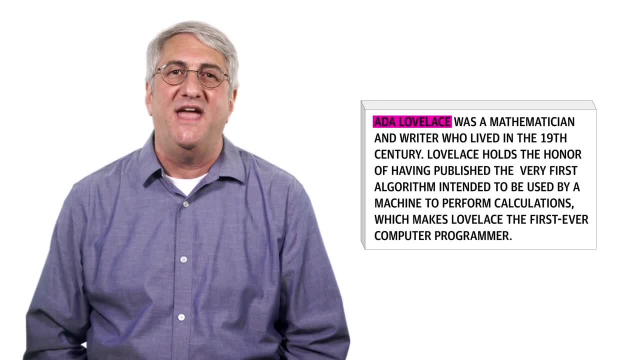 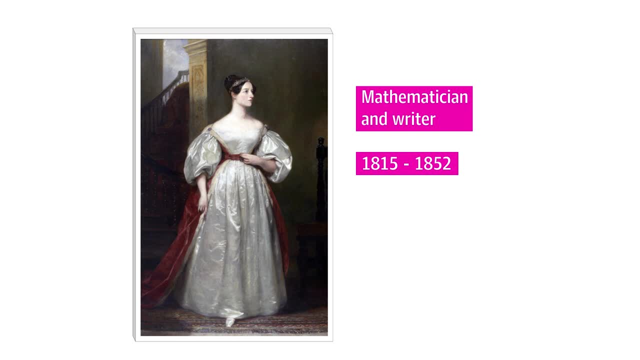 Giving infrared Bazooka. Let's say we're looking for the phrase Ada Lovelace in a paragraph. Ada Lovelace was a mathematician and writer who lived in the 19th century and she holds the Honor of having published the very first algorithm intended to be used by a machine to perform calculations. 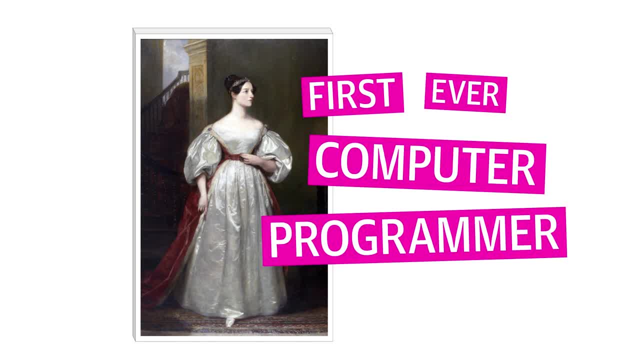 which makes her the first ever computer programmer In the first layer of the network. a CNN looks for the basic building blocks of an image, the basic building blocks of written language or letters. So what's the basic building blocks of one image? We sort of give it all an example, but we'll deal with that in just a short time, right? So if there's an example and there's an göster for 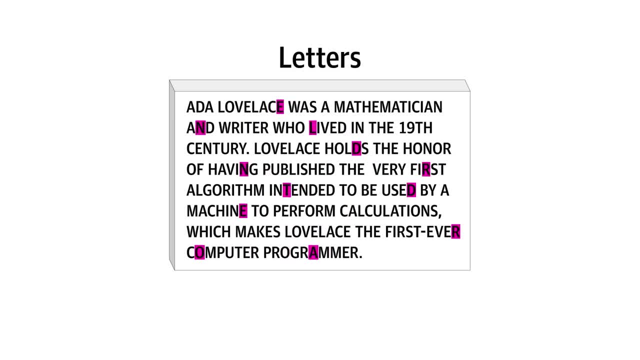 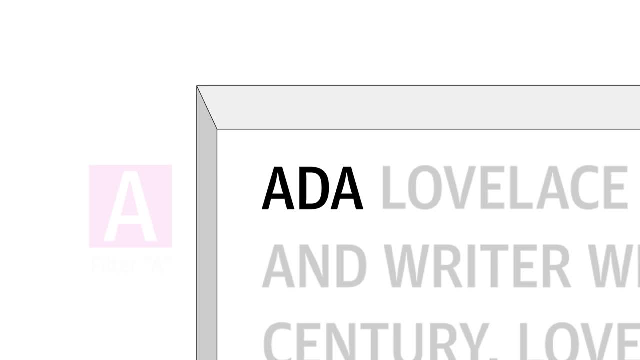 of written language or letters. so in this analogy, the filters the cnn uses in the first layer would be the letters. let's zoom in on the word ada. here's what the convolution process would look like for the letter a. when the a filter overlies the letter a in the original image, the convolution. 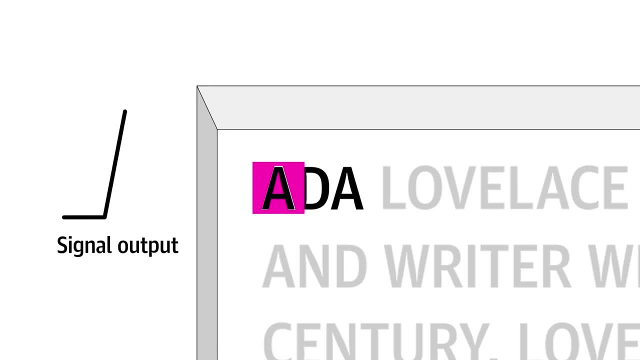 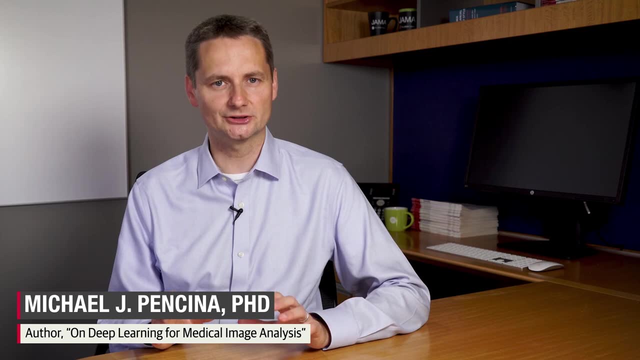 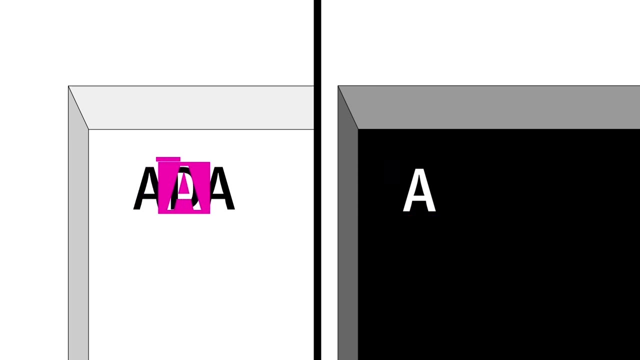 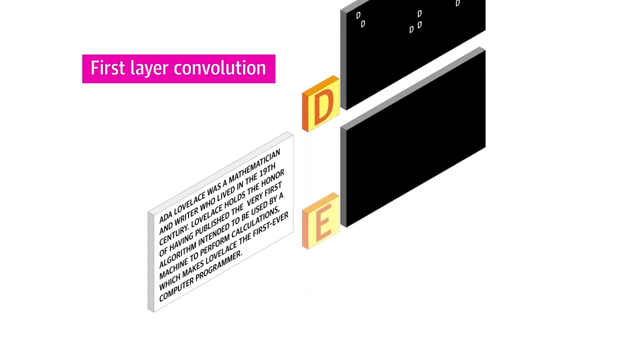 output would generate a strong signal. this signal would then be mapped onto something called a feature map. the feature map represents how well elements in the image align with the filter. if something is there, the signal outputs white. if nothing is there, the signal outputs black. cnn's generate a feature map for every filter. so in our analogy there would be a feature map. 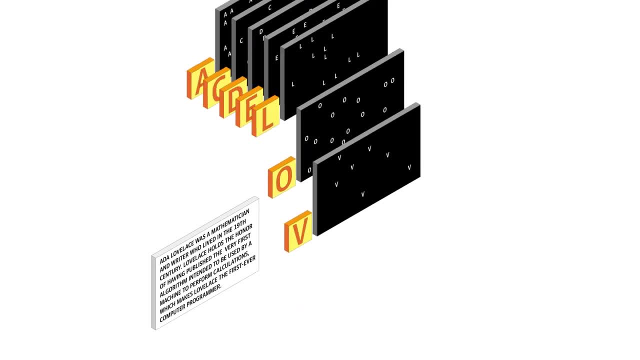 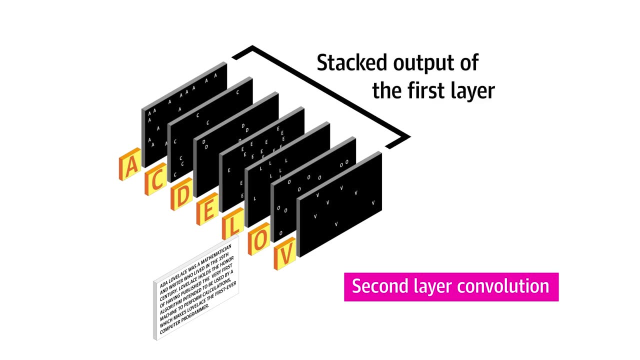 for every letter. these feature maps would then become the input for the second layer. in this layer, the cnn would spatially align and stack all those maps from the previous layer. this would allow the cnn to then look for short, specific sequences of letters in all the feature maps. 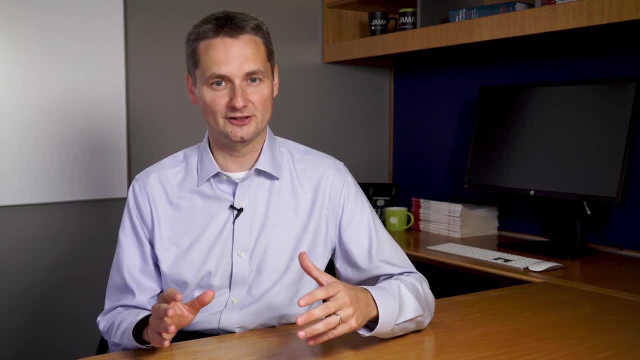 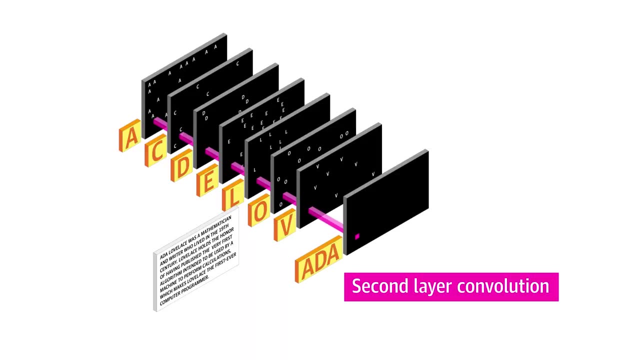 simultaneously. so the cnn would use a new set of filters to look for specific letters that are adjacent to one another, in particular sequences in our analogy. the second layer would look for places where the letters a, d and a are in sequence together, making the word eta. it would also look. 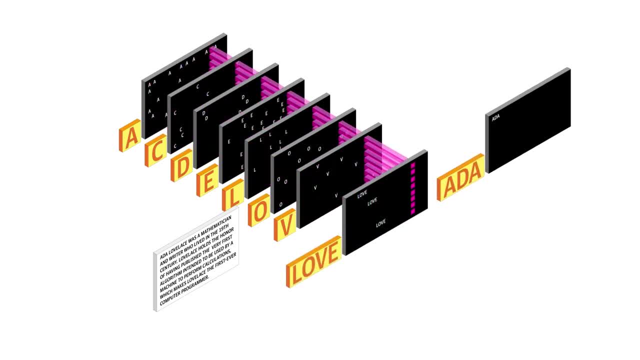 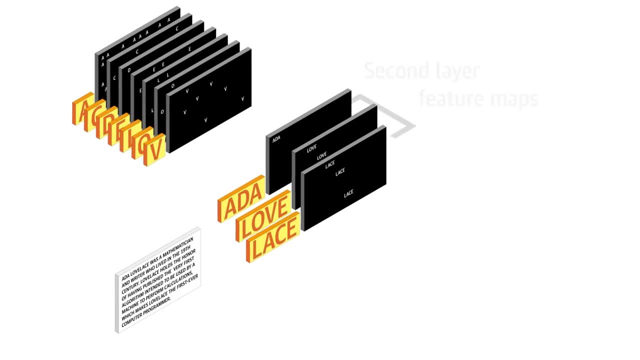 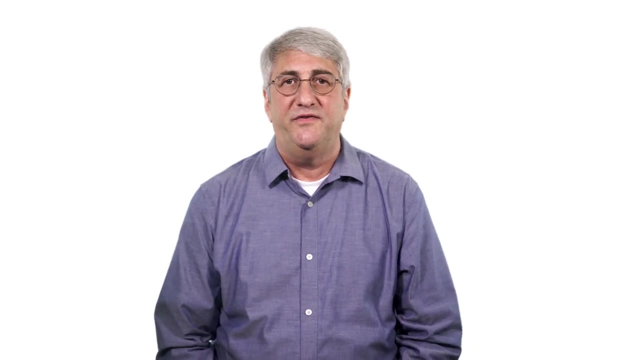 for places where the letters a, c, e, l, o, v are adjacent to one another, using filters for love. and the second layer would be the feature maps for those three sequences of letters. in other words, in those feature maps, strong signals would be present where the sequences ada, love and lace are located in the original paragraph. 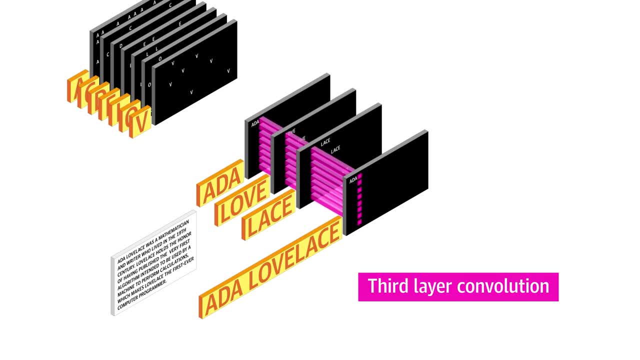 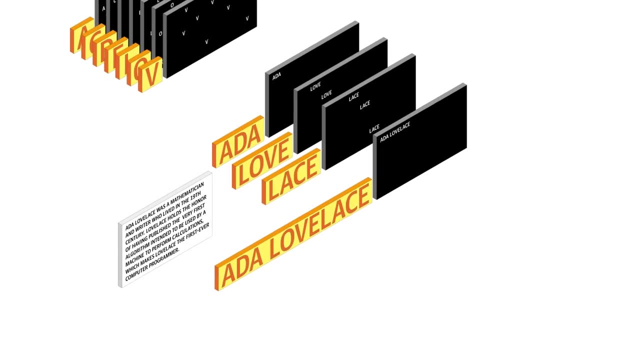 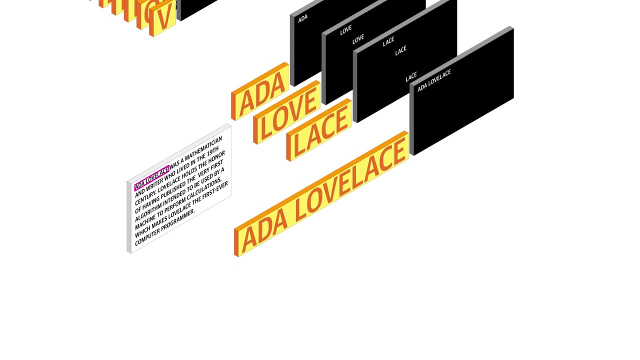 in the third layer, the cnn would stack and align these three new maps and perform more convolutions, this time identifying where longer words and groups of words are located. so the cnn could at this point identify where, in the original paragraph, the sequences of letters and words making the phrase ada lovelace are located. in our analogy, we were looking for a phrase consisting: 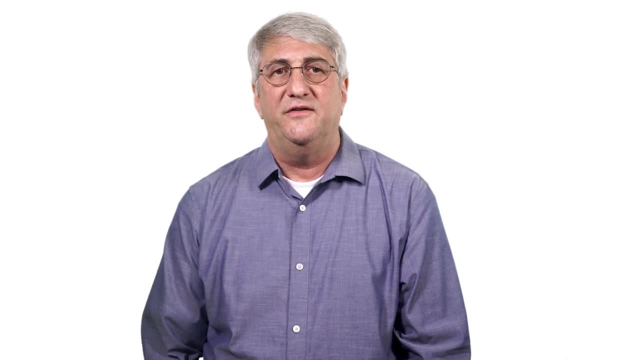 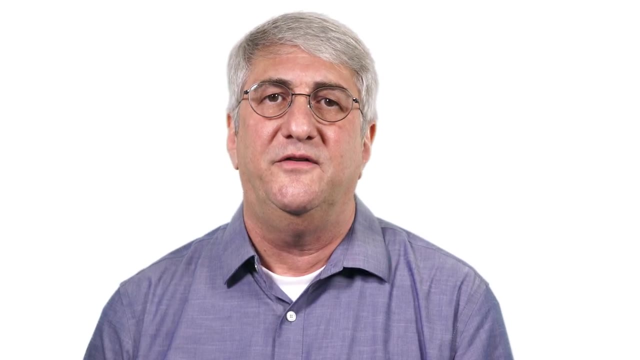 of only two words had we been looking for a longer sentence or even a paragraph? the cnn would deal with greater complexity by having more layers. we've omitted quite a few details about cnn's for simplicity, but this captures the essence of the model. but what does this look like for? 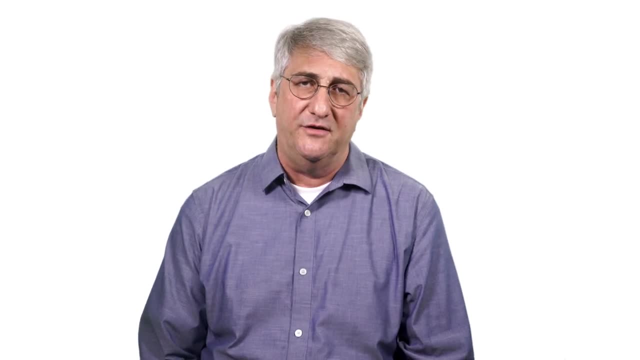 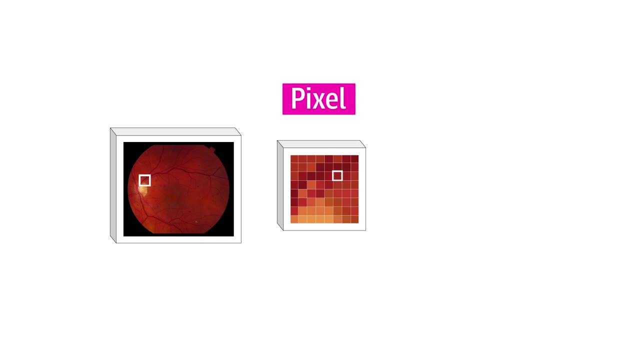 actual images, like identifying diabetic retinopathy from an ocular photograph. images are made out of rather than letters. in a digital context, a pixel is the smallest controllable unit of an image represented on a display. each pixel is a representation of a tiny portion of the original. 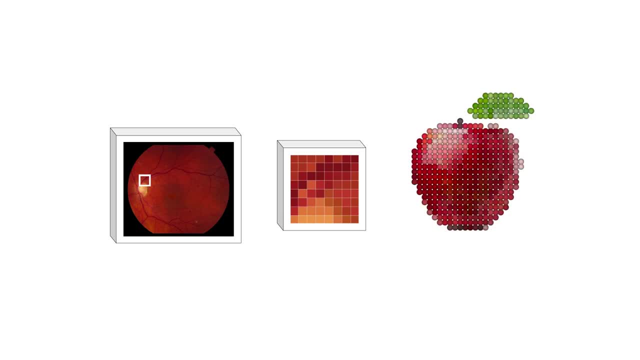 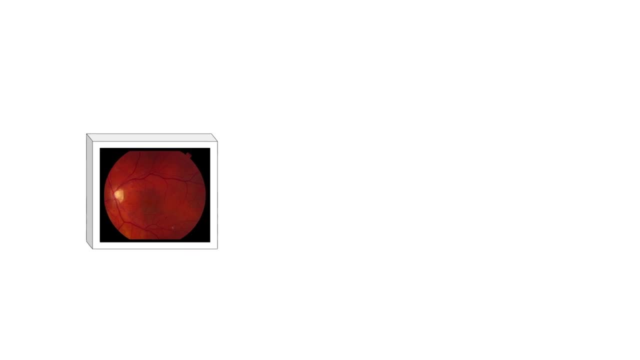 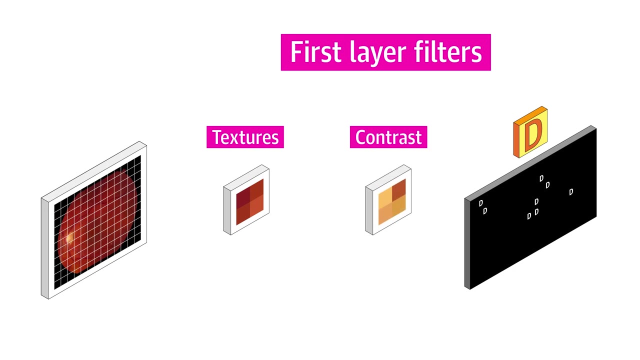 image. think about pixels, like creating a drawing with dots, where every dot has a color value and an intensity. the more dots used, the clearer the image becomes. the filters a cnn uses in that first layer are small squares of pixels that correspond to things like textures, contrast between two colors. 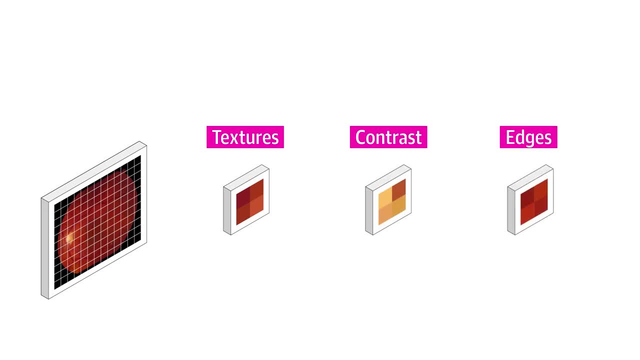 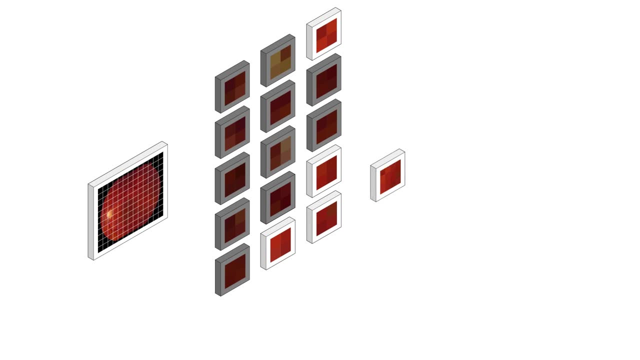 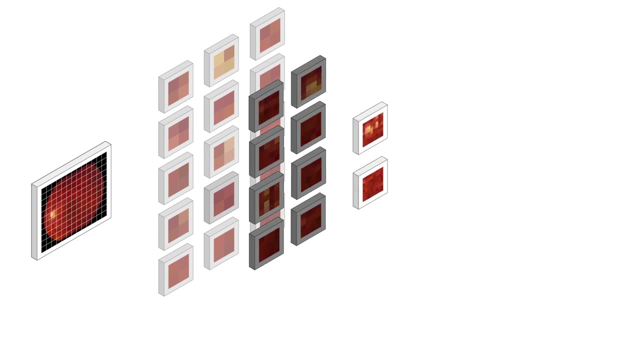 or edges. these are the image analysis equivalents of the letters used in our analogy, and as a cnn goes up in the hierarchy, it looks for combinations of these filters, getting more and more complex with each layer. as the complexity increases, the cnn gets closer to identifying what it's looking for. so the specific features analyzed at each layer help put the whole thing together. 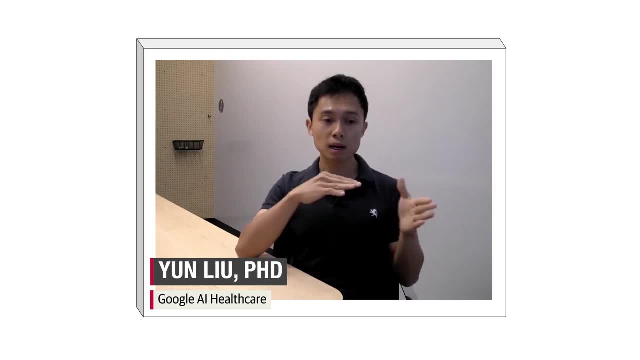 so, for example, some of the earlier work showed that some layers tend to be better at extracting sort of like edge length information, meaning that, for example, if we combine different kinds of horizontal edges, we might get a, a continuous line that resembles the retinal blood vessels, and as you combine more of those, you might start to encode more higher level concepts, such as 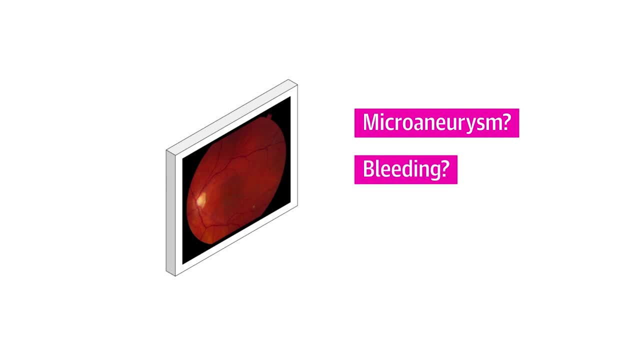 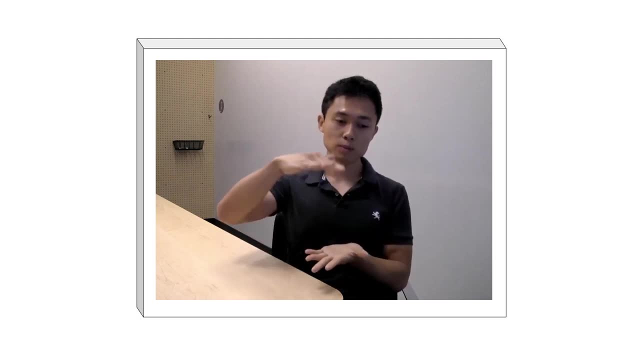 you know, is there a microaneurysm here, is there bleeding over here, is there other lesions in the image? and right at the very end is where these, after these multiple layers, the network will try to then condense all of that information down into a final prediction in. 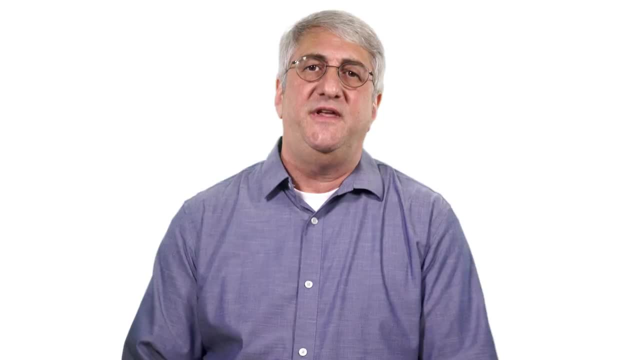 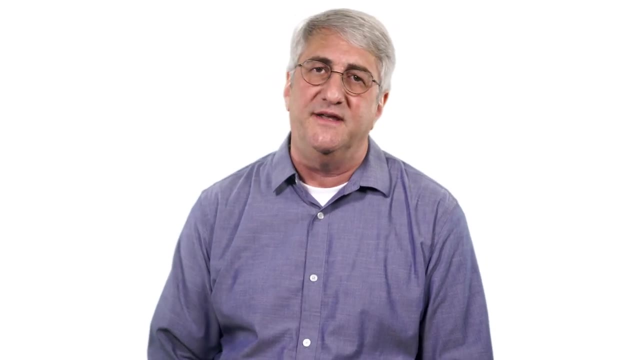 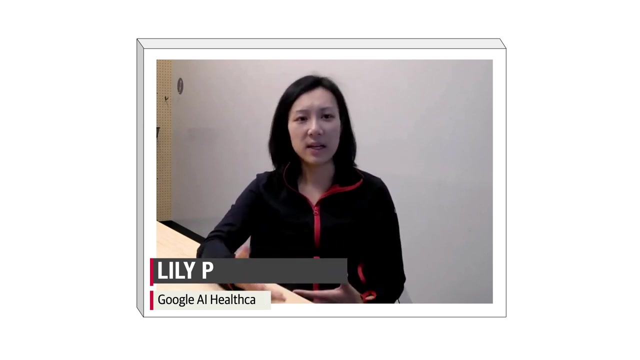 this case, severe diabetic. developing a cnn to help identify diabetic retinopathy was motivated because many patients with diabetes are not getting screened frequently enough. we have to screen diabetic patients once a year, or we should, and there are some barriers to getting that done. some of it is just, you know, not having enough trained professionals to do that task. it's also 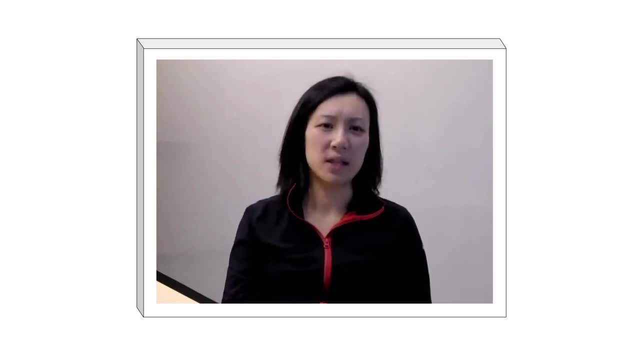 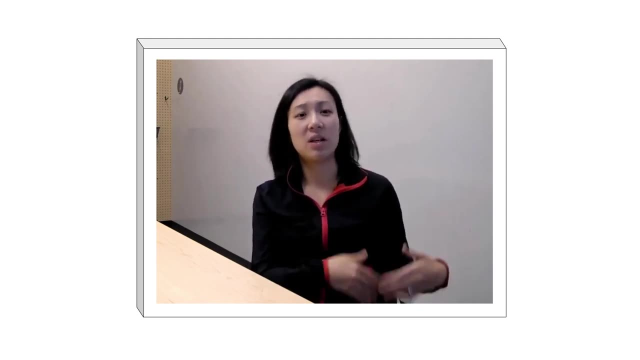 to not having that expertise available where the patient is. It's not that you know there aren't retina specialists in a metropolitan city four hours away. It's that there isn't a retina specialist at your grocery store, And CNNs would facilitate the integration. 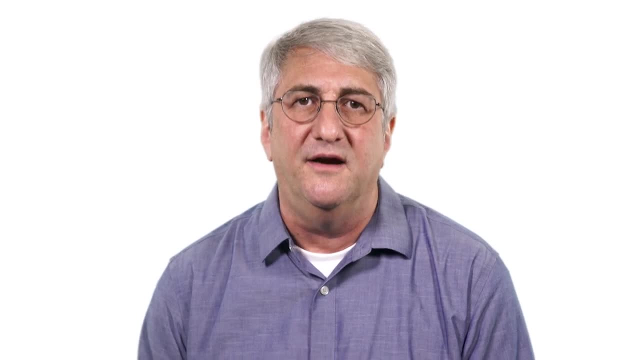 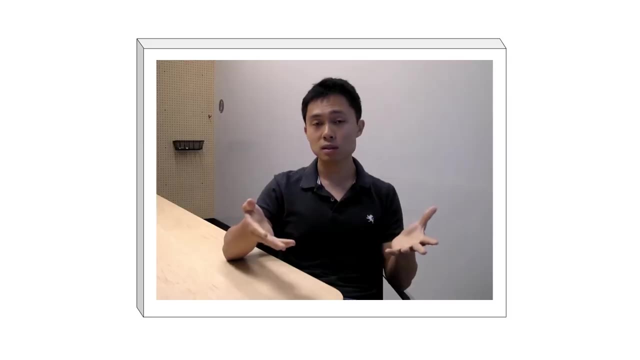 of diabetic retinopathy and other screening programs into primary care. But before that happens, more research, especially prospective clinical trials, are needed. The way we do approach these things is really the way that medicine usually works, which is to say, let's do validations of the method. 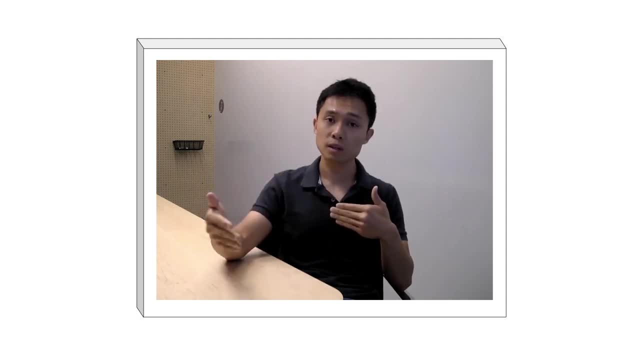 again, and again, and again, until we're sure we're, you know, reasonably confident that it really works on many kinds of images in many settings, for you know many different patient populations, And so from my perspective, that's really, end of the day, what's most important. 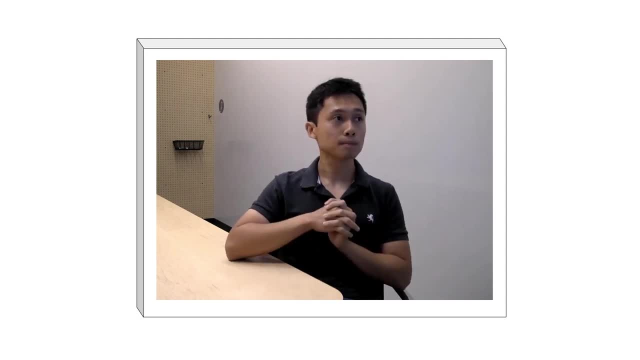 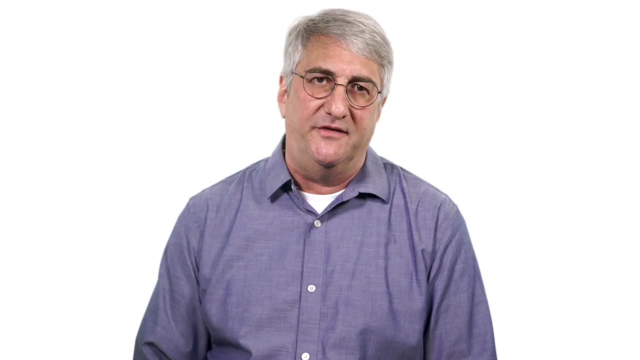 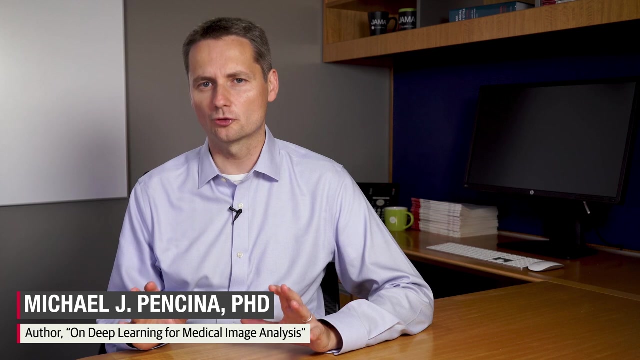 Does it work on real patients and is it reliable? The excitement generated by early results has already spurred several research groups to look into the efficacy of CNNs in clinical practice, Which could potentially finally get CNNs from the bench to the bedside. I think we're on the third or fourth. 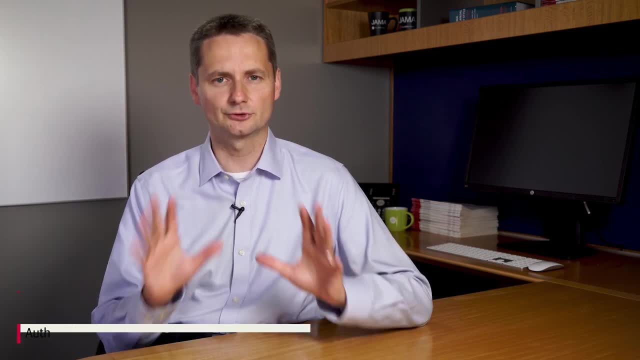 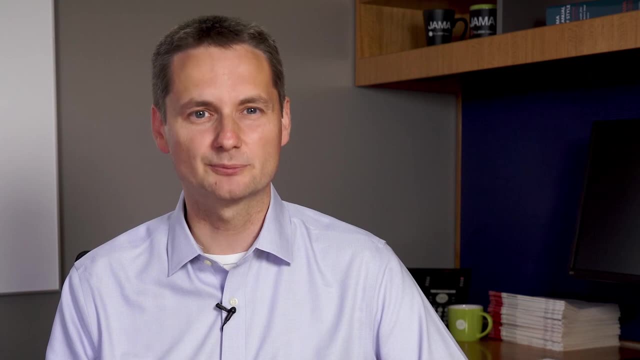 technological revolution where neural networks are coming to the forefront, And I really hope that this time we'll get it right. But there were failures in the past where people used technology in suboptimal ways, and we don't want it to happen again. One has to make sure that we have appropriate 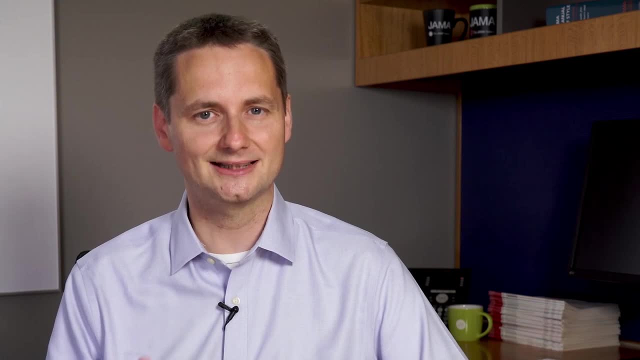 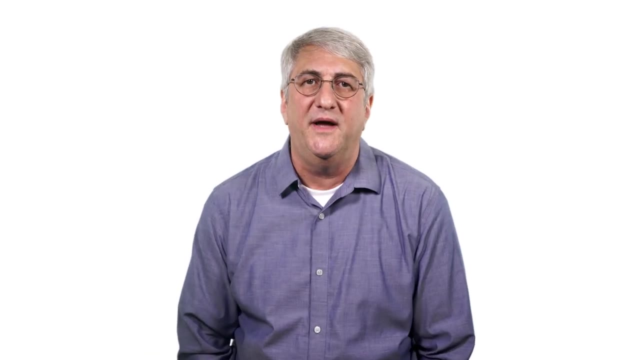 and sufficient data for development, validation and testing, and that we're solving actual clinical problems. At the end of the day, one thing to take away is that, even if, as a clinician, it can be hard to understand exactly how CNN. 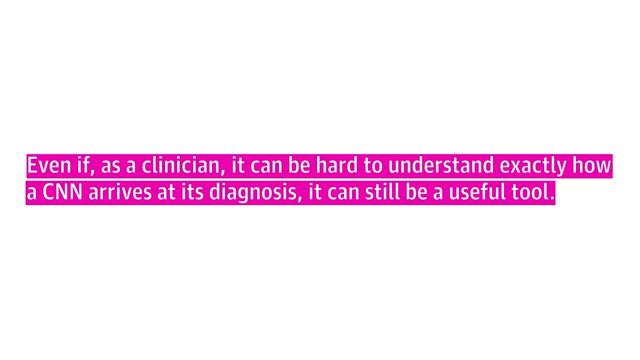 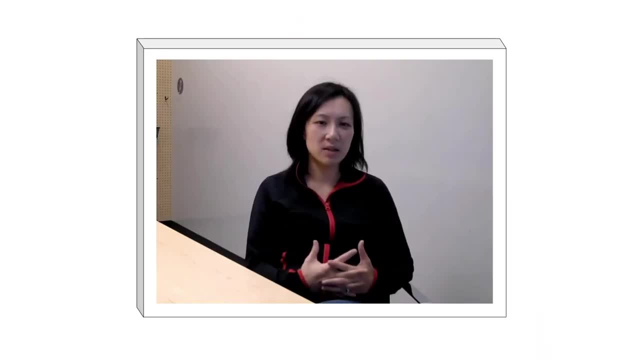 arise at its diagnosis, it can still be a useful tool, And this is similar to how many clinicians use other widely adopted technologies. Consider antibodies: You know, as a clinician I may not know exactly where that part of an antibody kind of binds to. 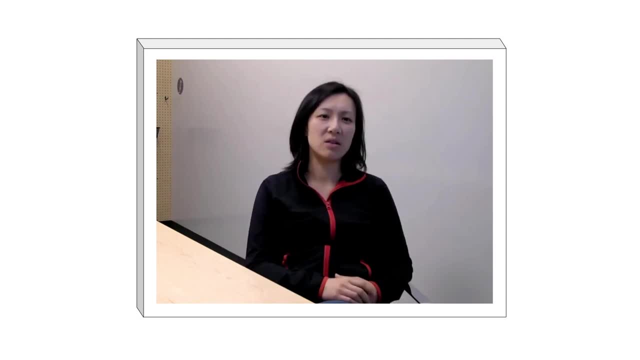 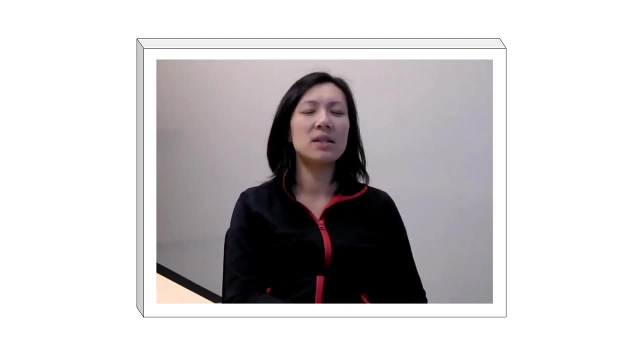 but I'm comfortable after looking at some of this clinical validation of using Lucentis, for example, for an injection right. This is kind of like any new breakthrough technology needs validation and needs transparency. But I think you know the medical community in general.